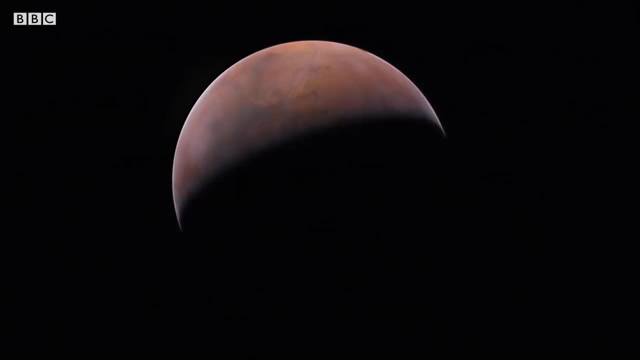 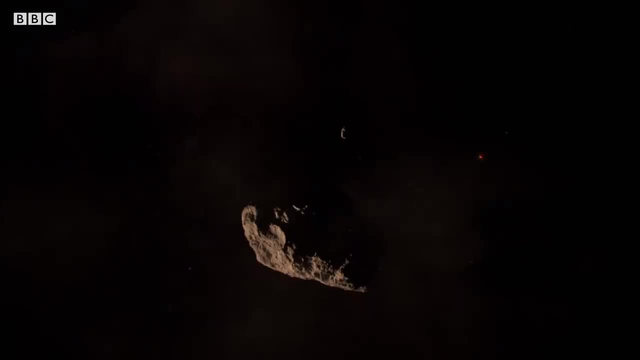 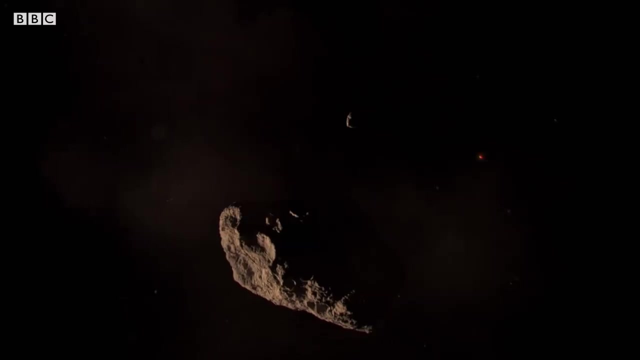 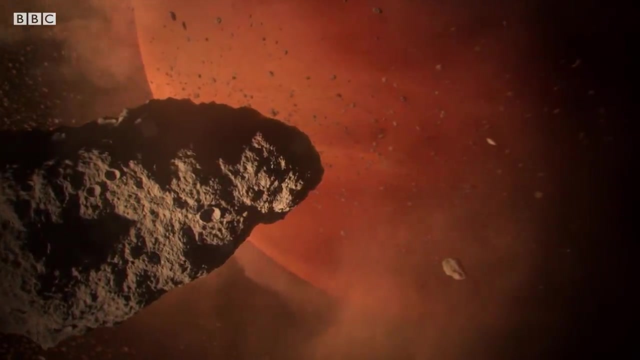 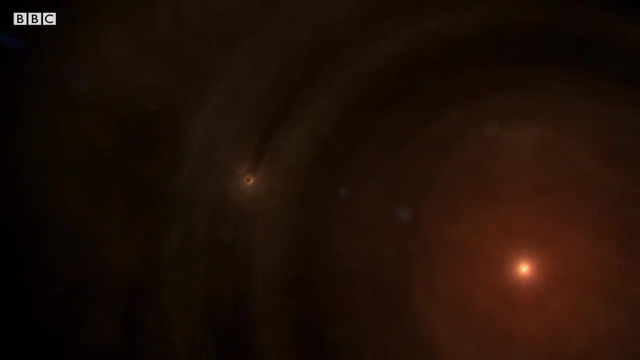 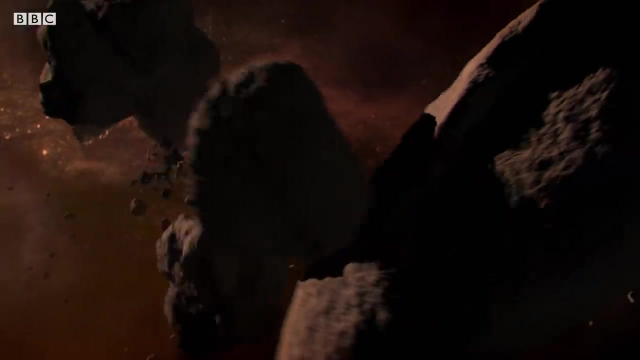 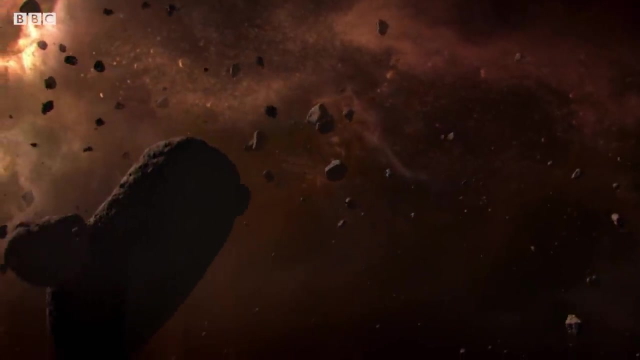 Mars would suffer a similar fate at the hands of Jupiter. After marauding through what would become the asteroid belt, Jupiter enters the region of space where Mars is forming, Continuing its journey, spiraling towards the Sun As Jupiter bulldozes inwards. 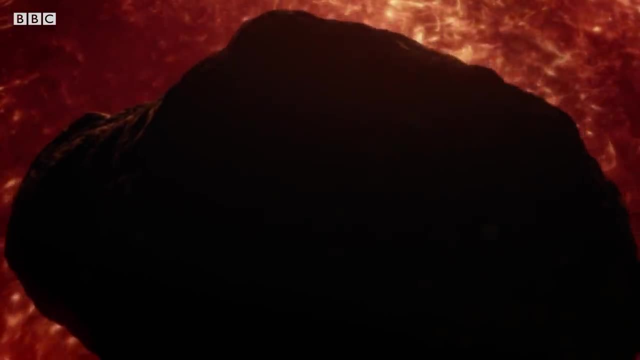 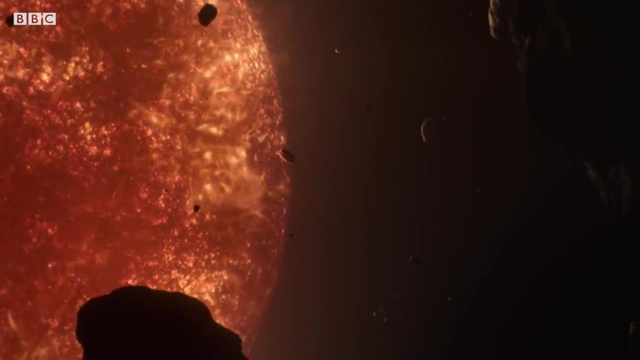 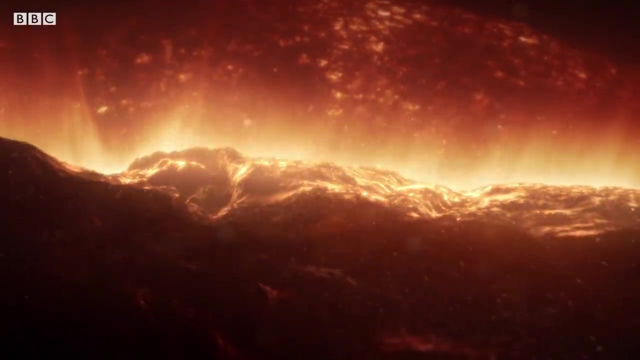 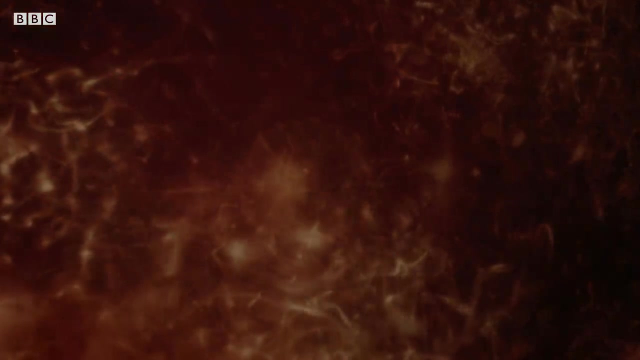 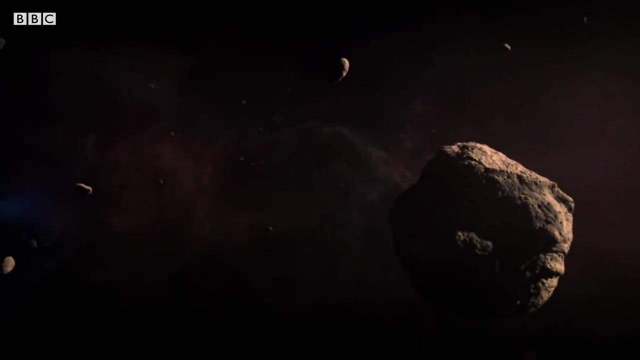 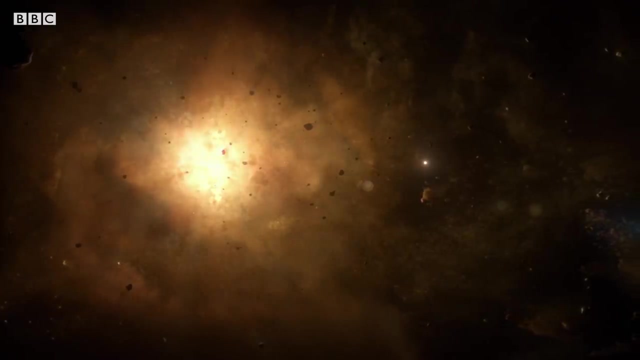 its immense gravity scatters material in all directions. Some is sent careering into the Sun And some is thrown out into interstellar space. It is because of the gravitational clearing of this neighborhood by Jupiter that Mars was unable to grow to more than 10% of that of the Earth. 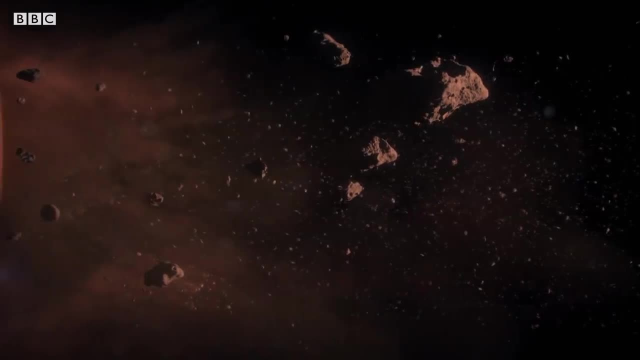 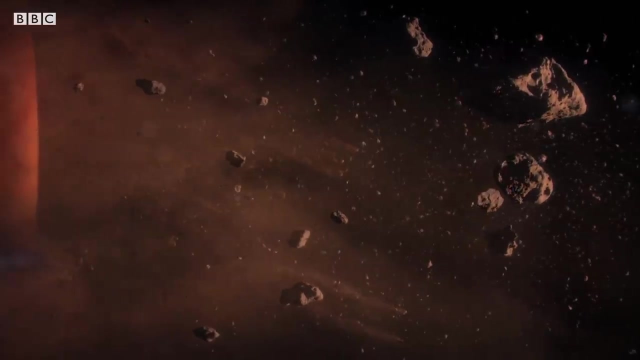 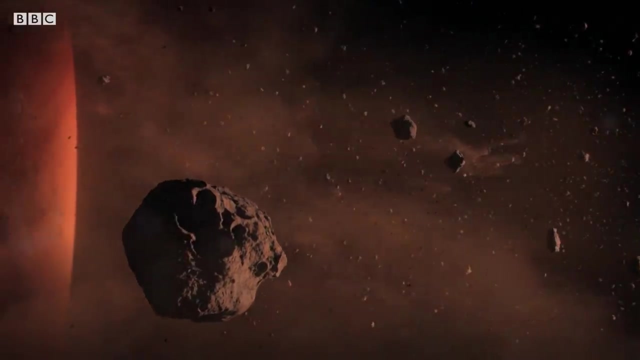 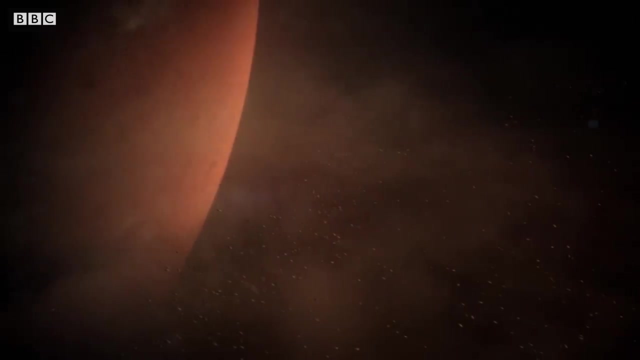 This is why Mars is small, And by clearing material out of the inner solar system, the giant planet may also have prevented the formation of the super-Earths we see in other systems, And if it had continued moving inward, our planet too might never have formed. 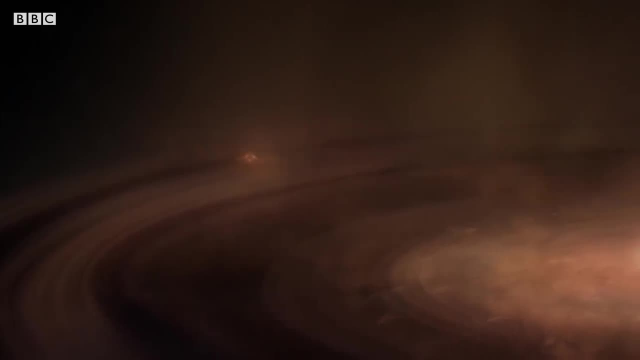 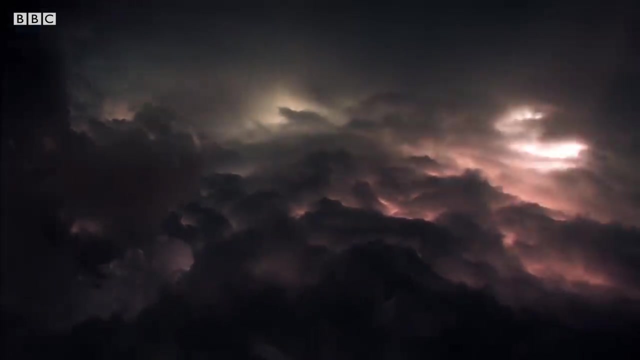 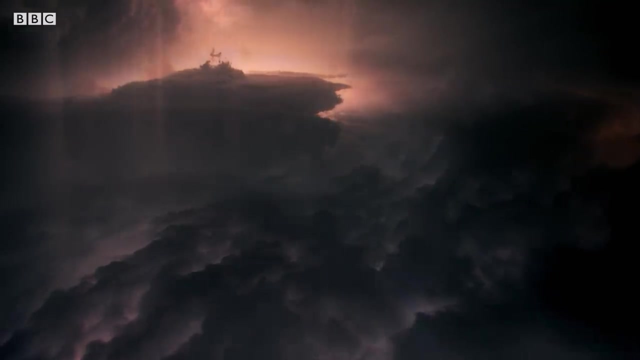 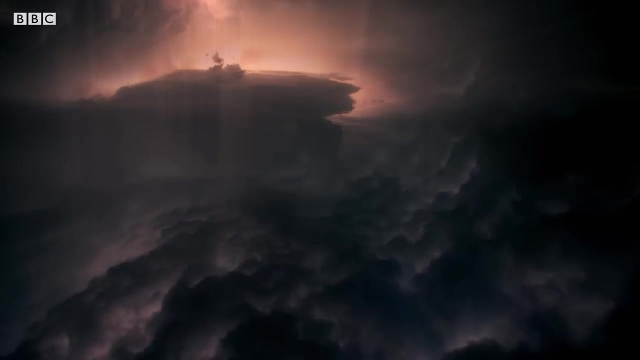 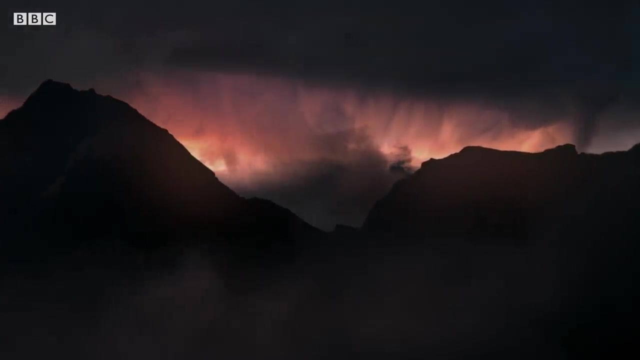 But then, just as it looks like, Jupiter will sweep everything away, the giant planet stops in its tracks Because, in the shadows of the outer solar system, another planet is forming, The solar system's second gas giant, Saturn, And its arrival changes everything. As Jupiter moved inwards, Saturn moved inwards and caught up to Jupiter's orbit. When this happened, the two locked into a special configuration known as a mean-motion resonance. This is where the planets begin to interact gravitationally in a very coherent manner. 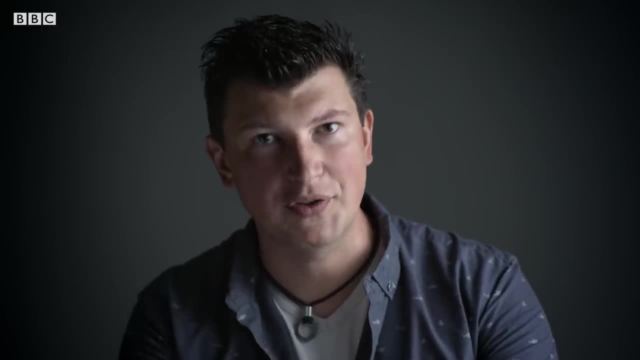 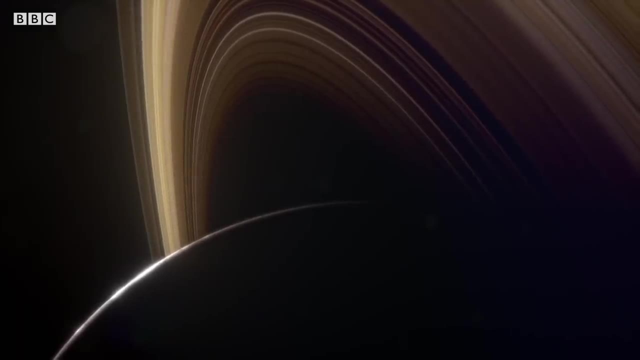 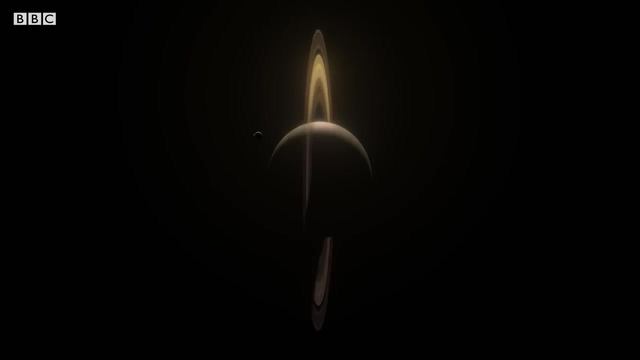 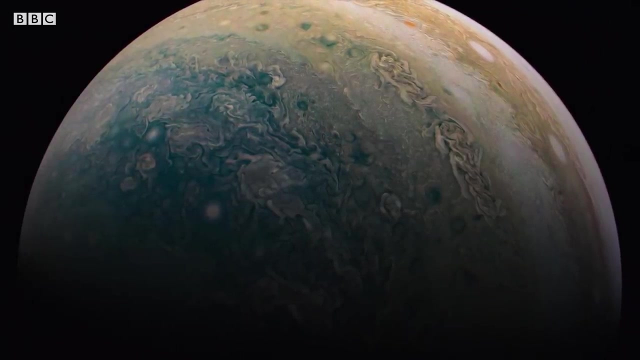 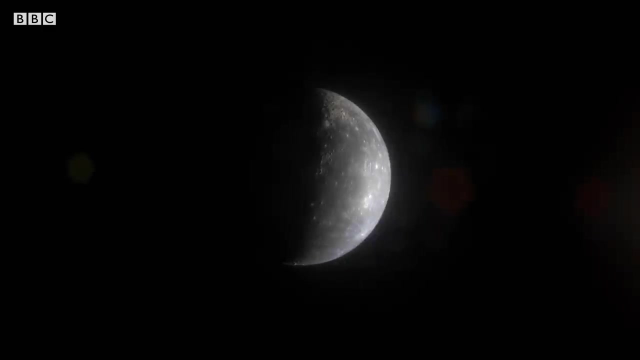 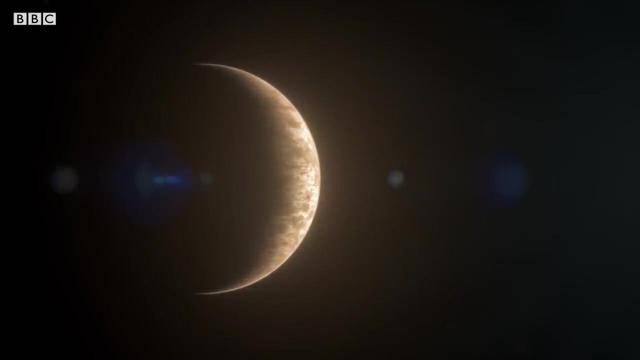 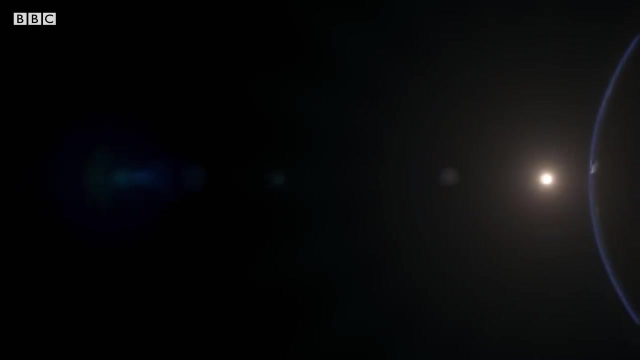 And now locked as a unit. the two reversed their migration course and moved back out. Saturn caused Jupiter to retreat, Leaving behind just enough material from which the inner planets could form. Mercury, Venus And our home Earth is in exactly the right location. 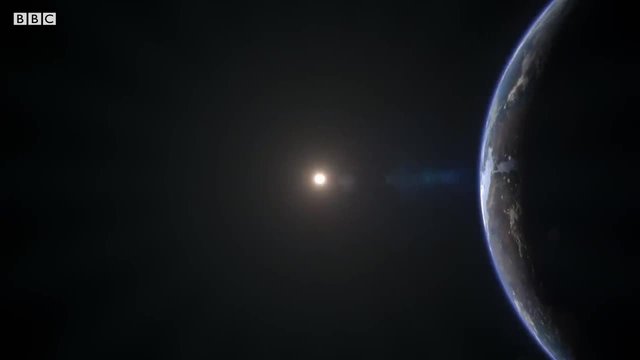 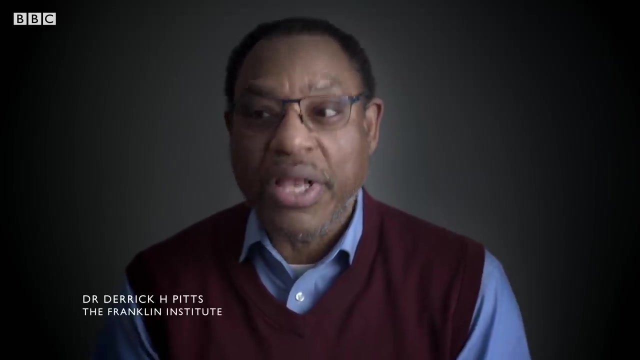 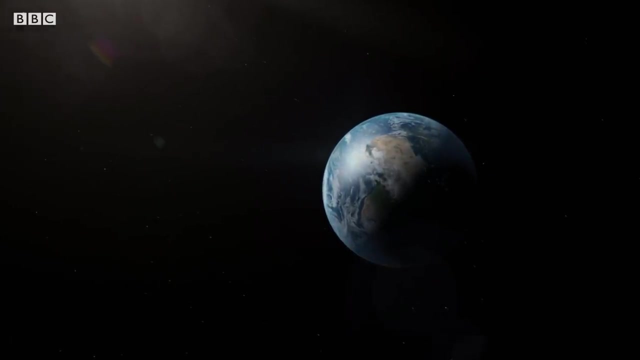 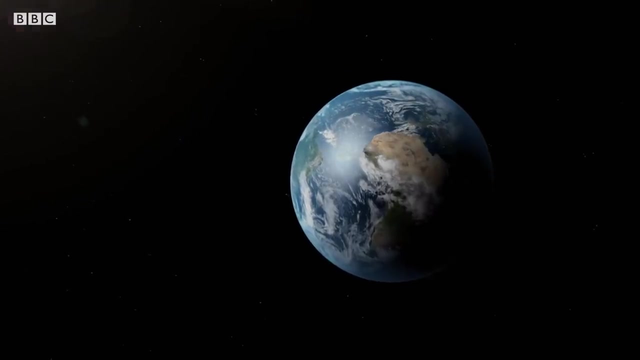 to provide the environment for life to develop. So if Jupiter had moved around even more, who knows, maybe life never would have developed in the solar system as we know it. And as its voyage across the solar system draws to a close, Jupiter helps to provide our living world. 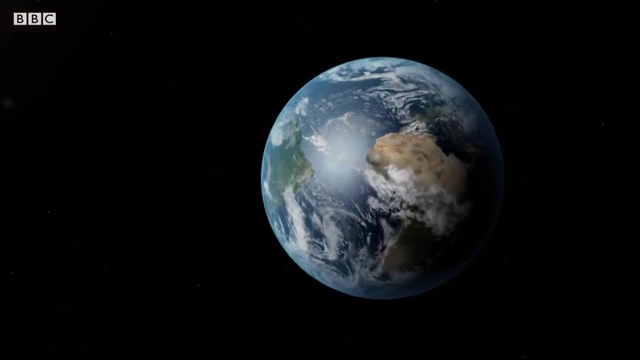 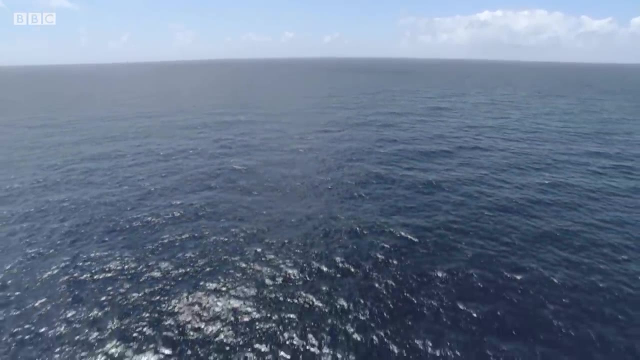 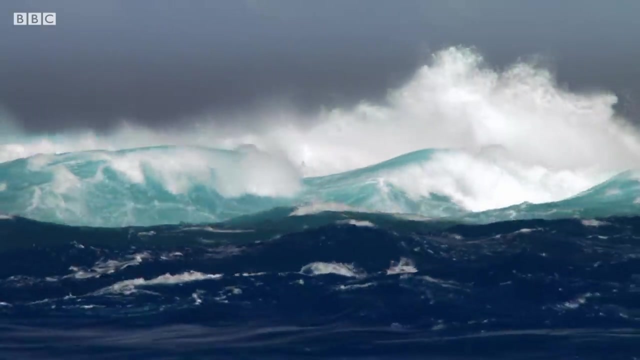 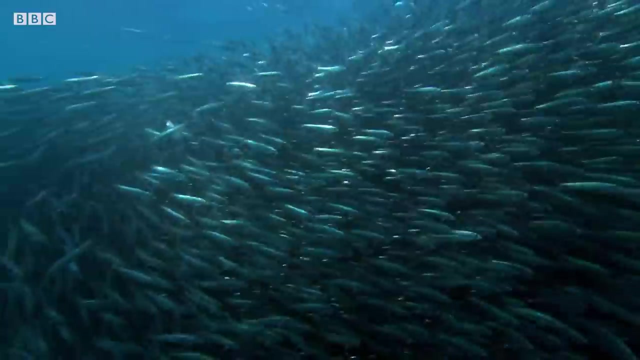 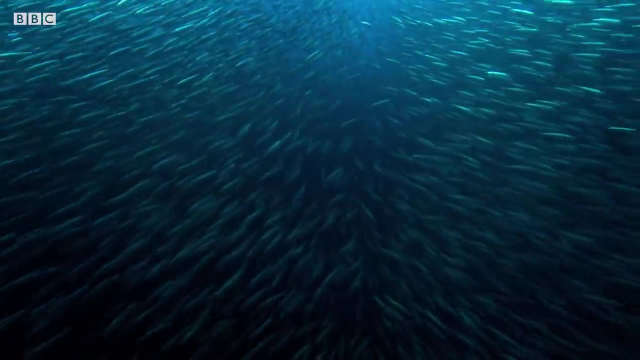 with its most precious ingredient: Earth. Today, two-thirds of our planet's surface is covered by ocean: More than 1.3 billion cubic kilometers of water Each drop, teeming with life. One of the big questions about the evolution of our solar system is 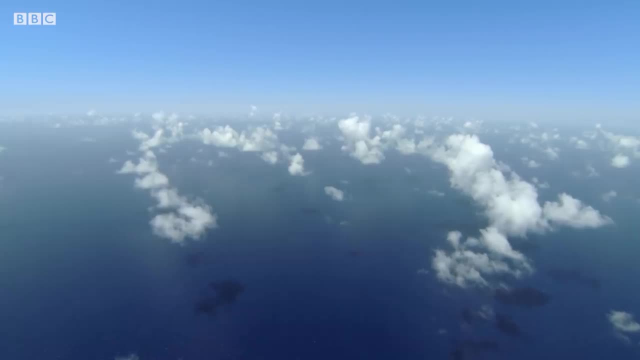 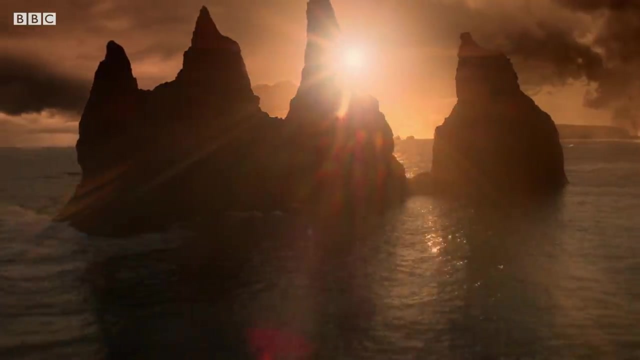 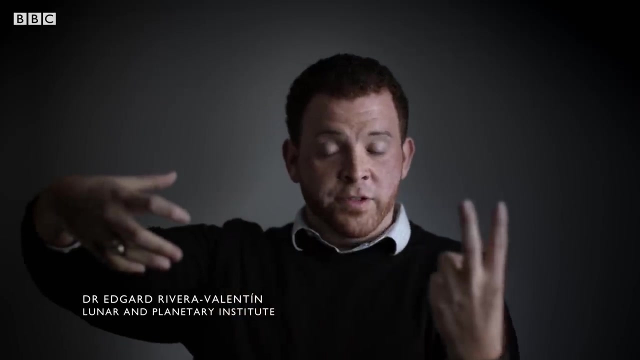 how did we get water here on this planet? So we think that the inner planets didn't naturally form with a lot of water. Water is primarily in the outer solar system, But if you end up having Jupiter and Saturn moving outwards, then that is able to suddenly deliver more water. 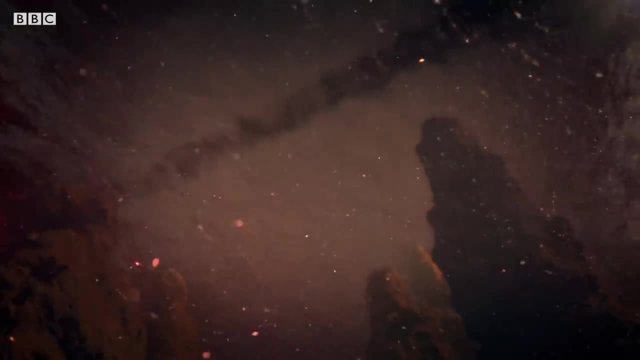 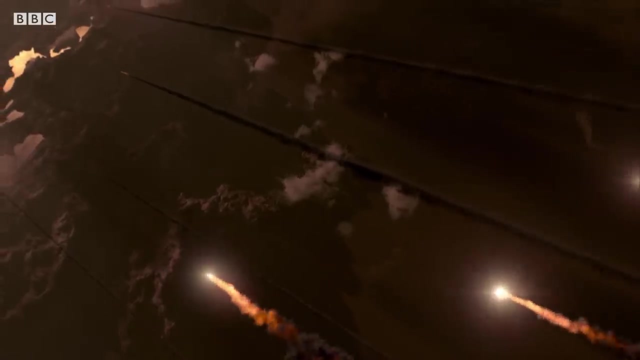 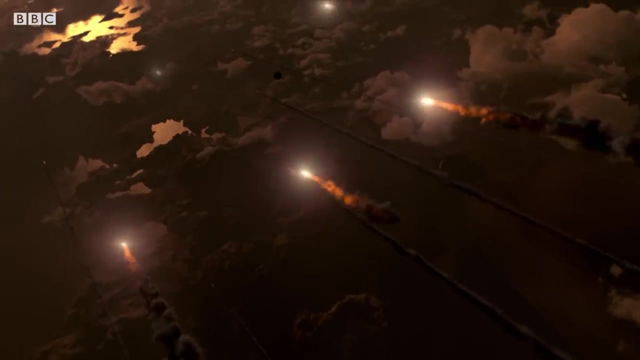 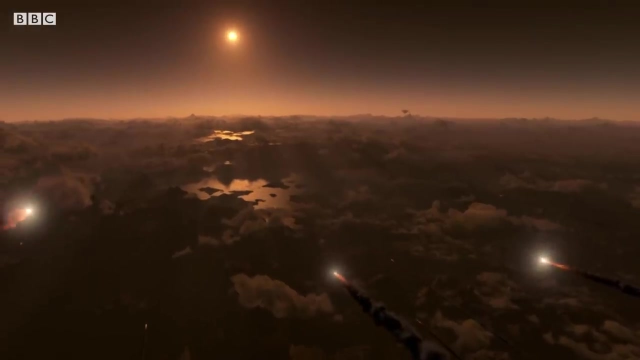 into the inner solar system. Locked in a gravitational dip, Jupiter and Saturn dance with Saturn. Jupiter moves back through the asteroid belt And as it does so, water-rich material is flung inward, where it is incorporated into the growing terrestrial worlds.